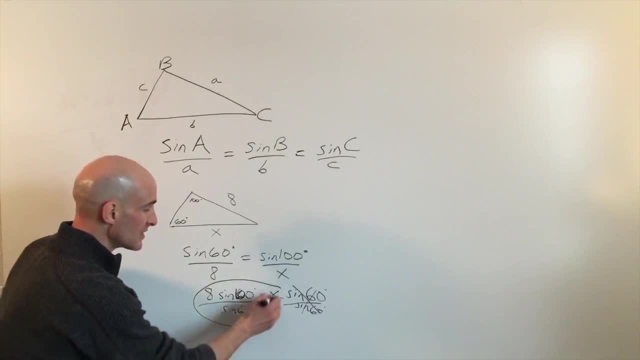 degrees. these are going to cancel you and X is going to equal that quantity right there. so let's just check real quick and see what that is on the calculator. so let's see my mode. let's see I am in degrees. okay, that's good. and let's see we've got 8 sine 100 divided. 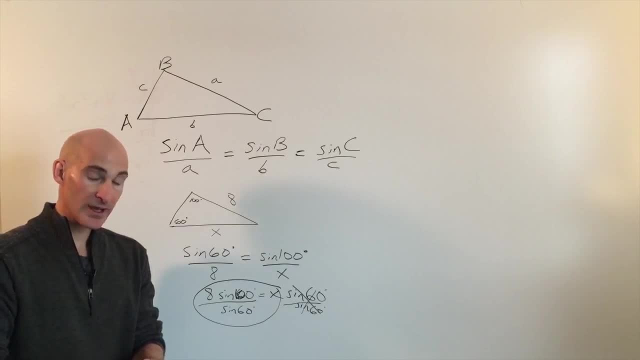 by sine: 60. okay, 9.1 approximately. okay. so that's the law of sines. now what comes up with the law of sines that often times confuses students is what they call the ambiguous case. so we're going to talk about the ambiguous case. this is where there can be two triangles there. 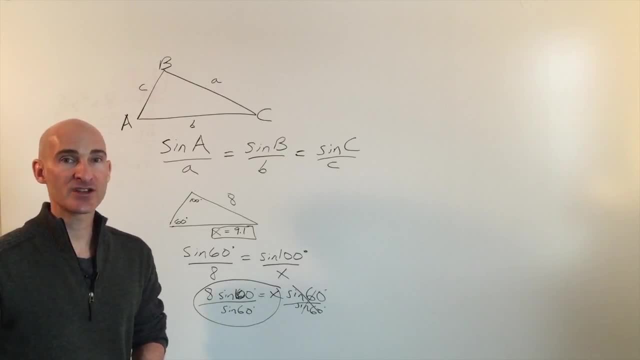 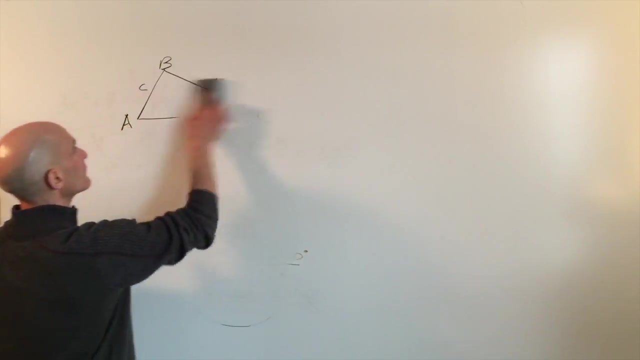 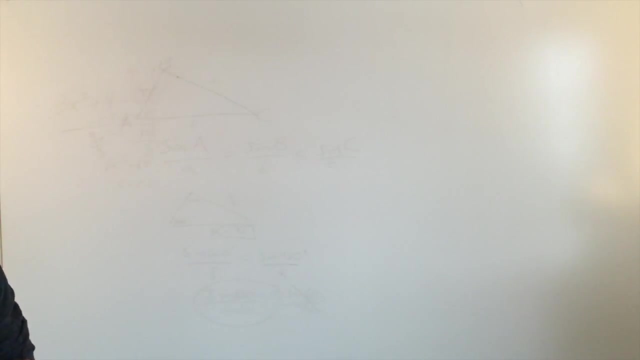 can be one triangle. there can even be no triangle, given the information that they give you in the problem. so let me see if I can show you how that works and let's take a look at that. you, you, you, I'll show you how that works. okay, so when you do the law of sines, the 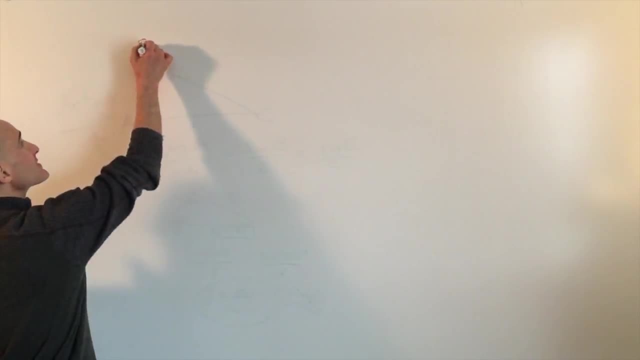 ambiguous case. it occurs when you have side side angle, and the reason I wrote it like that is because this is going to be an acute angle. the side next to that acute angle is going to be longer than the side across from that acute angle. so I'll show you what I mean. 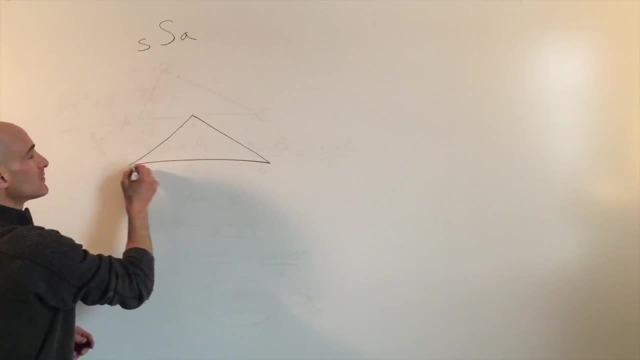 so say, for example, this is 30 degrees, and say this is 10, and say this side over here is 6. okay, what you want to do is you want to drop an altitude like that? so now what we have is we have a right triangle right here on the left and we're going to find 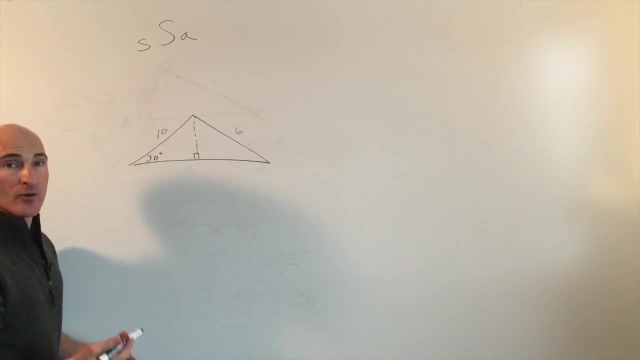 out. what is that altitude? so to do that, we're just going to use regular right triangle trigonometry. sine of 30 degrees equals- I'll call that h- h over 10. so sine of 30 equals opposite right partners. what you can do is you can cross, multiply on the diagonal and you get. 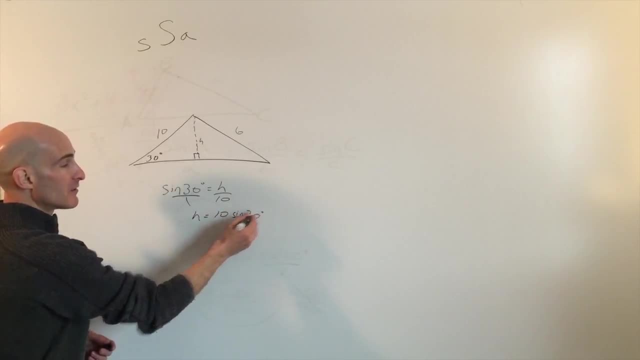 h equals 10 times the sine of 30 degrees. sine of 30 is a half times 10 is 5. so this height is 5. okay, now here's where the analysis comes in this side, right here. we don't know anything about this angle. okay, we don't. 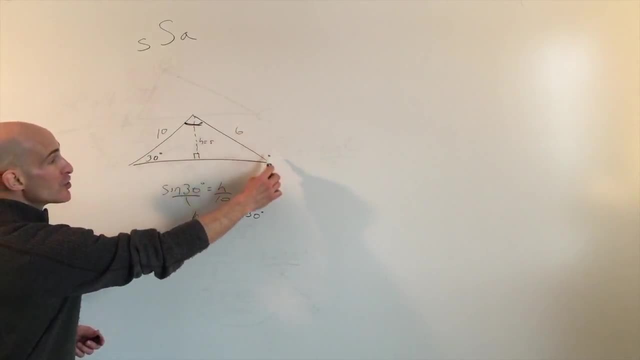 know anything about this angle, this side here you could rotate the side in such a way that it could actually be like that. so you could rotate it. so this triangle can even could either be like this or you can rotate it like that, because we don't know what this angle is, it's not fixed, so what we end up here in. 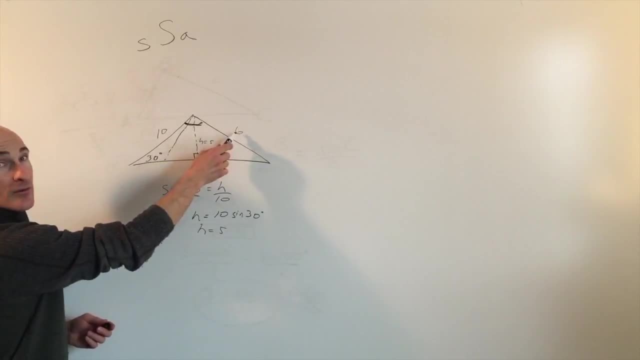 this situation where this side across from the acute angle is in between the altitude and the side adjacent, that's when you get two triangles. Okay, now say, for example, this side over here, instead of being six, it was four. 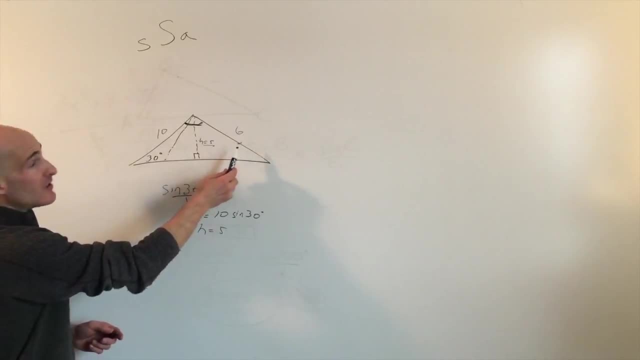 Well, if it was four, it would only be like this long right here, And if you rotate it, so you think of this as a hinge- if you rotate it, it's not going to be long enough to reach this side, So in that case there would be no triangle possible. 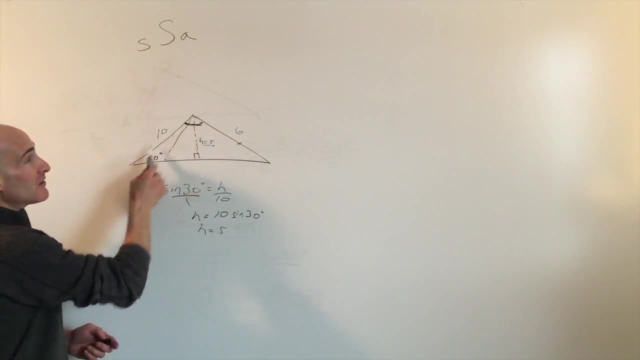 Now, if this was exactly five, it would be a right triangle. If this side was greater than ten, again, think of this as a hinge. if it was greater than ten, if we swung this side over here, it would be too long. 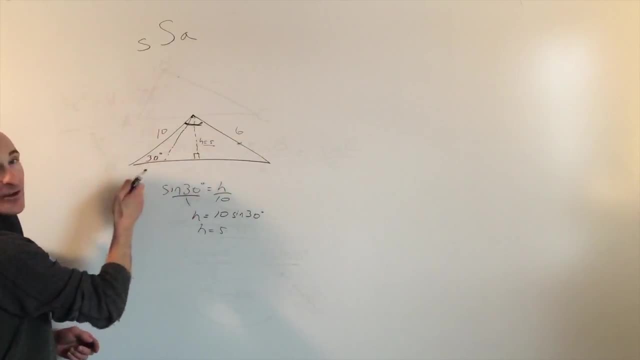 It wouldn't intersect this side. It would actually go past this side right here. So in that case you're just going to have one triangle possible. It would have to swing out like that. So these are the different cases with the law of sines. 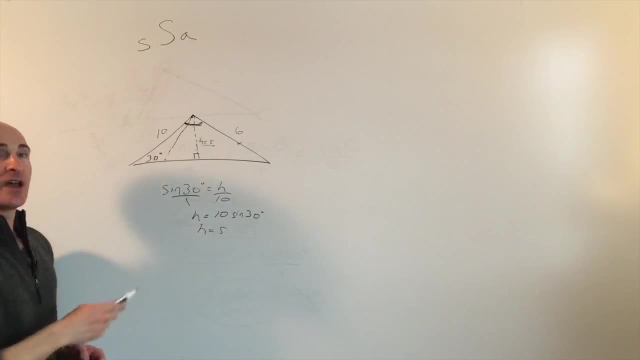 Let's take a look at how to solve this problem that has two, Two triangles, and then we can look at some other examples. So the first thing you want to do is let's label this triangle A, B and C. 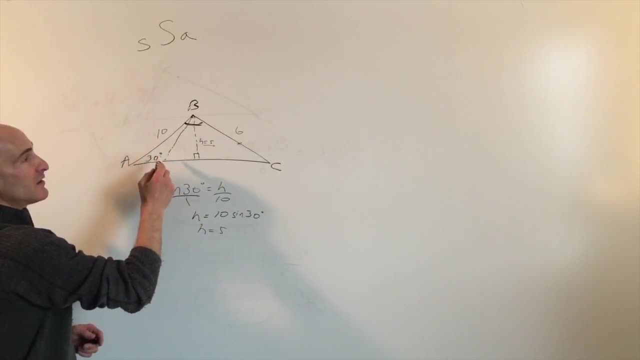 This is going to be side A, side C and side B across from each other. So what we're going to do here is we're going to do the law of sines: Sine of 30 over 6 equals sine of C over 10.. 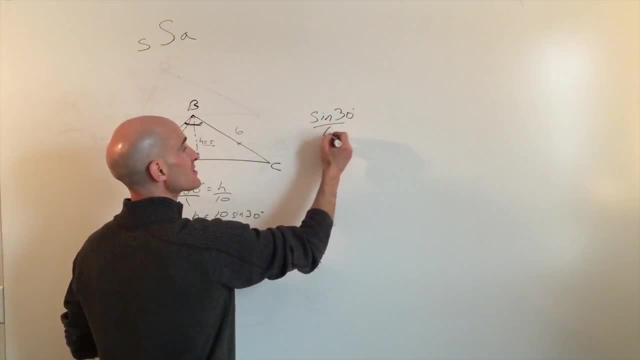 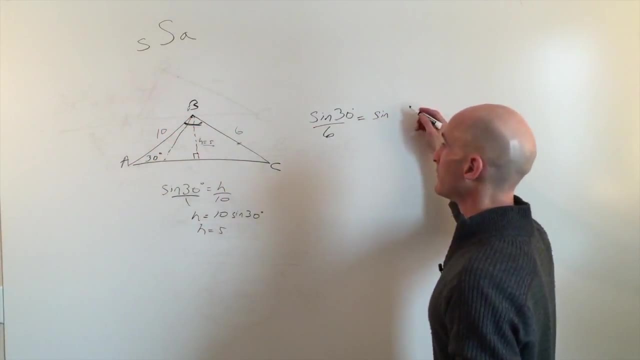 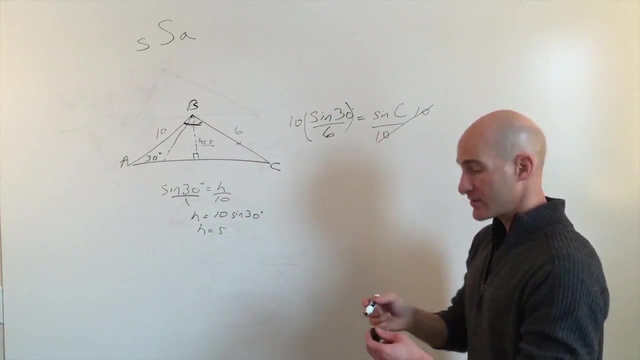 Sine of 30. Over 6 equals sine of. go to this side here. sine of C over 10.. So again, if we multiply both sides by 10, these 10s are going to cancel. And if we simplify this on our calculator, let's see what that comes out to. 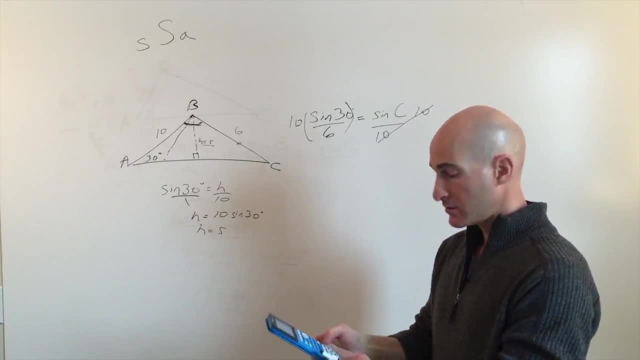 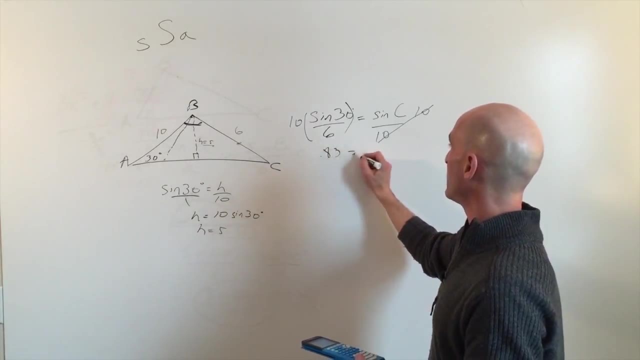 10 times the sine of 30.. 10 times the sine of 30, divided by 6, 0.83.. So I'm just going to round: 0.83 equals the sine of C, And then if you take the sine inverse of both sides, that's how you solve for angle C. 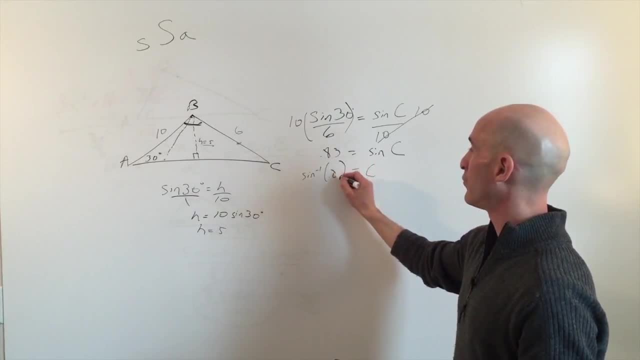 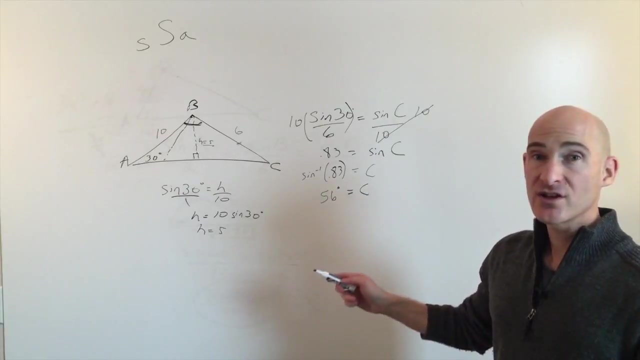 So C is the sine inverse of 0.83.. Let's do that Sine inverse 0.83.. We get 56.4 degrees. Let's just call it 56 for this example. Keep it simple. Now, what I want you to realize is when we took this side here and we swung it like this: 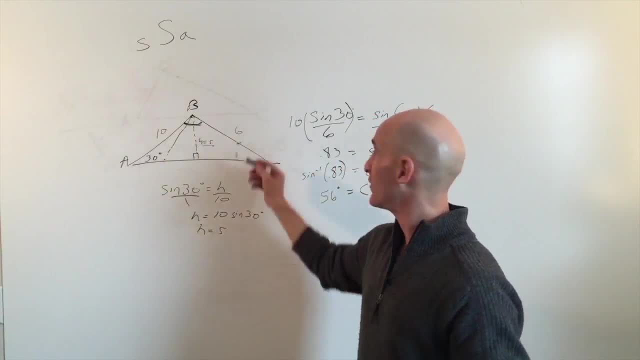 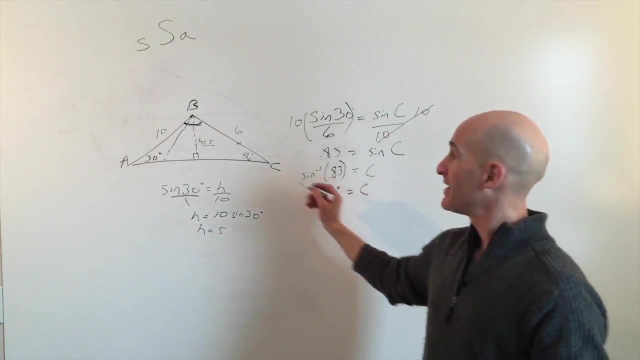 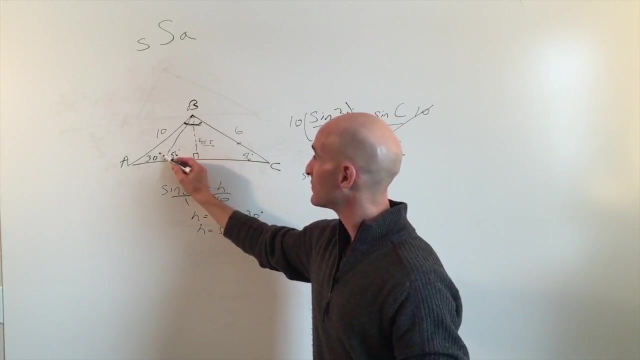 this actually forms an isosceles triangle. So if this is 6, this is 6.. If this is 56 degrees, which we just solved for this here will also be 56 degrees, And by doing 180 minus 56, we can solve for this angle right here. 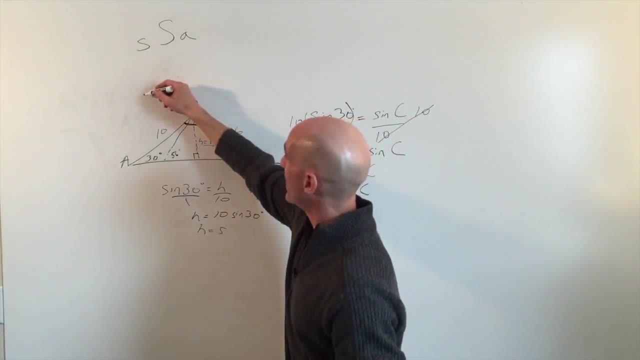 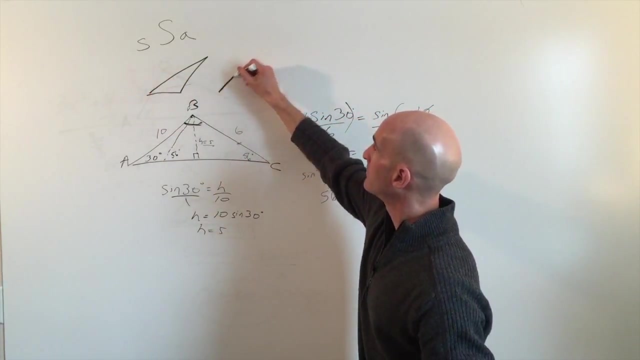 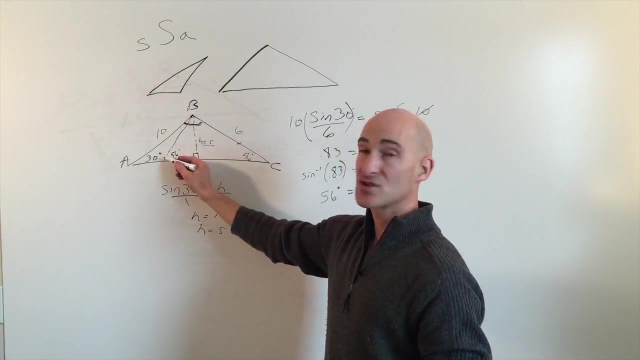 So what we've got here is: we've got this triangle, Okay, that's this one right here, And we have this as a possible triangle right here. So if this is 56, this would be 180 minus 56, which is 124.. 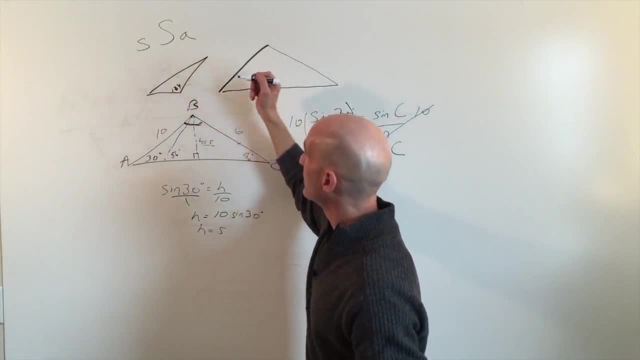 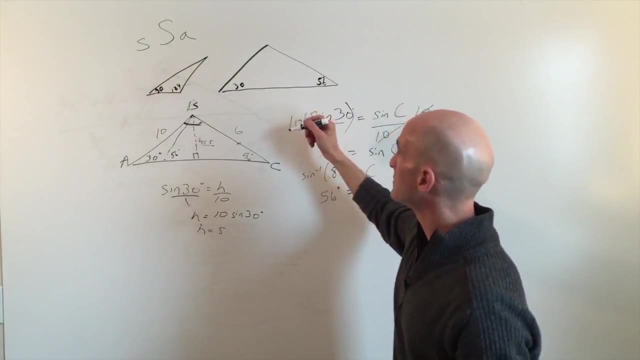 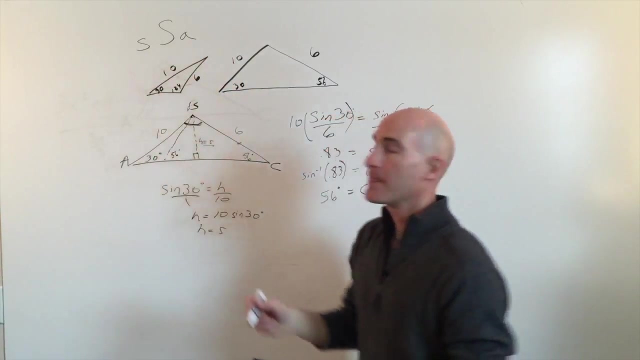 So this is going to be 124.. This is 56.. This is 30.. And this is 30. And What else do we know? This is 6.. This is 10.. This is 6.. This is 10.. 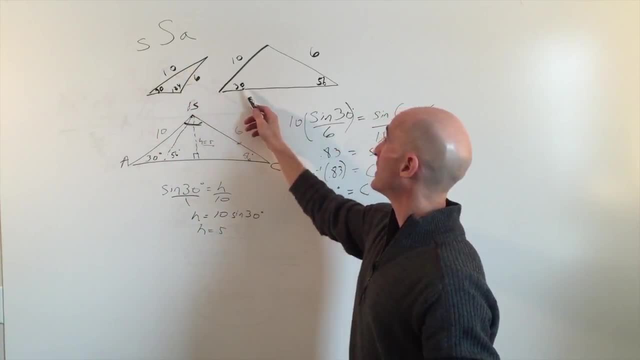 And so now what you can do is: you can add these two angles together and subtract from 180 to find this angle. You can add these two angles together, subtract from 180 to find this angle. So let's do that. That's 86.. 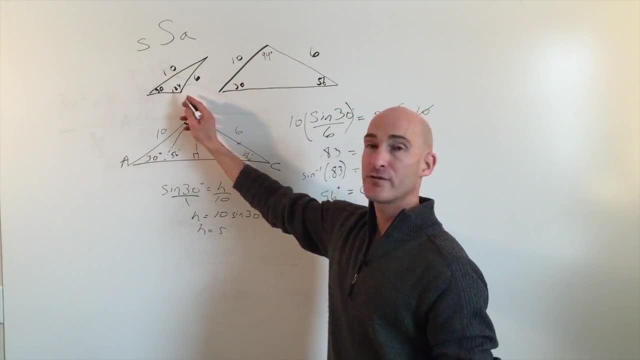 So this must be 94. This one here is 154.. Which means this must be 26.. Okay, Okay now, what you're going to do is you're going to solve for this missing side right here by doing the Law of Sines again. 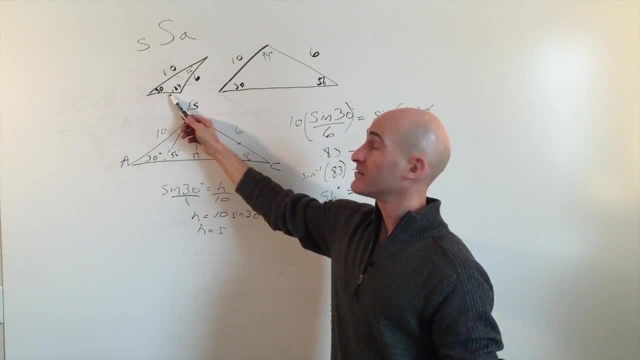 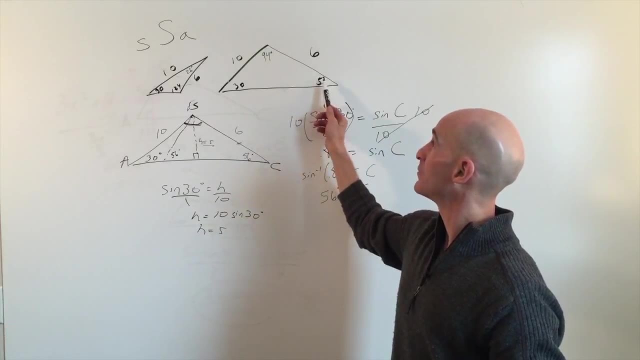 So sine of 26 over the side opposite equals sine of 30 over its side opposite. Same thing here: Sine of 94 over its side opposite equals sine of 30 over its side opposite. And that's how you're going to solve for these two missing sides. 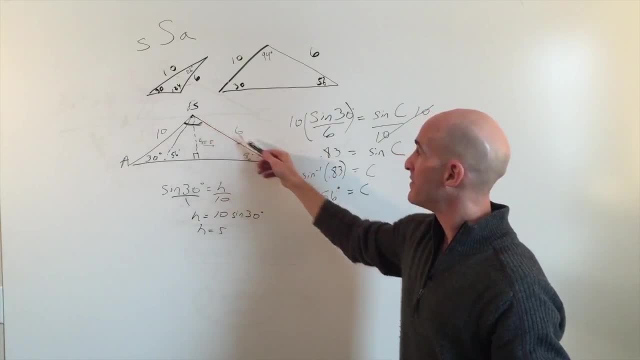 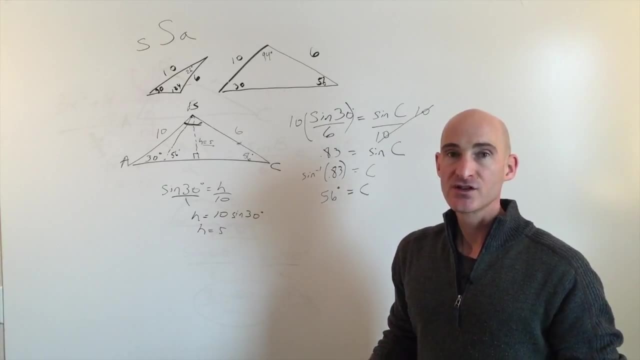 So in this case you get two triangles And again that's because This side Was in between the altitude and the side adjacent, So there's actually two possible triangles. So that's the Law of Sines, The ambiguous case. 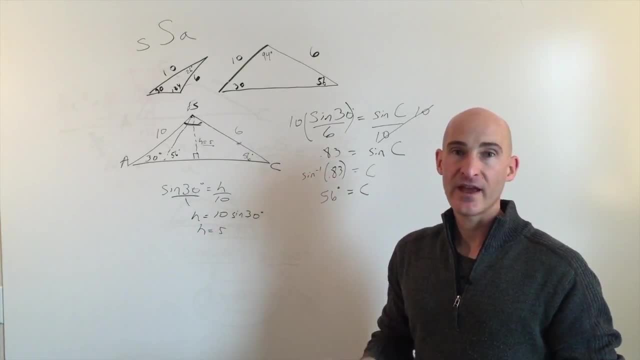 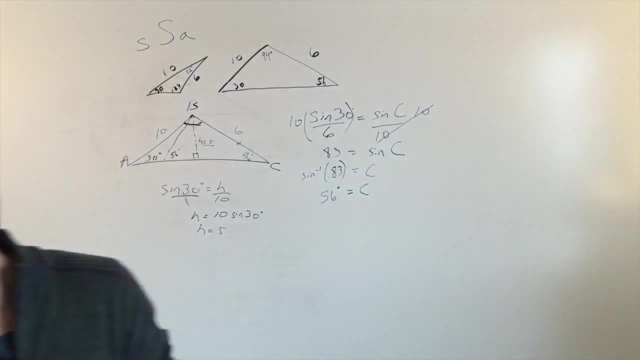 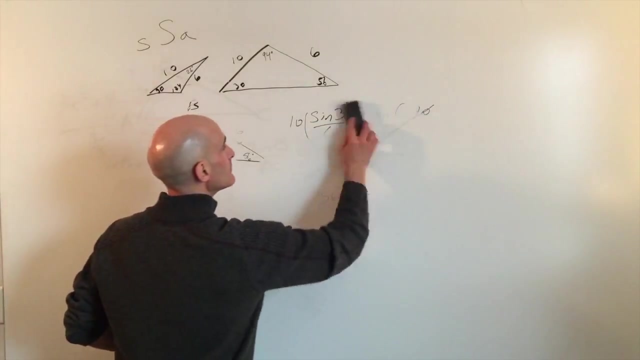 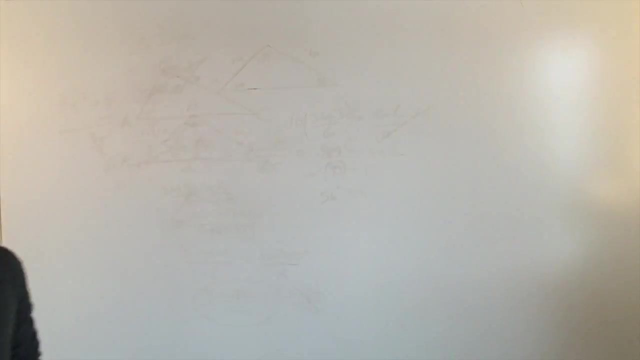 And now what I want to do is just talk a little bit about how to find the area of a triangle, if it's not a right triangle, if you don't have the altitude, And let's just take a look at that next. Okay, so what we're going to do is we're going to find the area of a triangle. 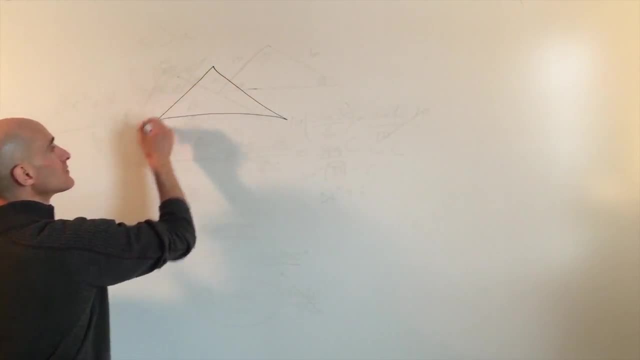 So say, for example, your triangle is like this: Say this is 10.. Say this is 70 degrees, Say this is 15.. Okay, You want to find the area of the triangle. Now, before we learned, the formula for the area of a triangle was what? 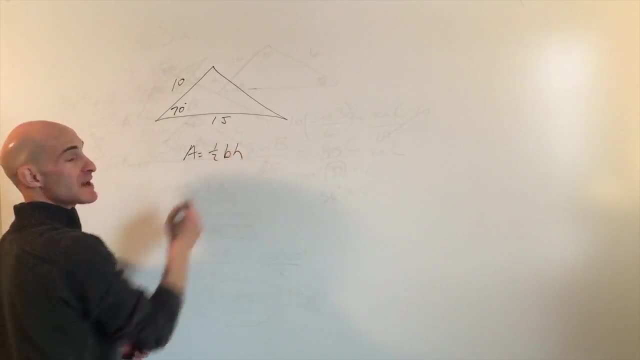 1 half base times height. The base is the bottom, The height is this right here. Okay, the altitude, That's how tall the triangle is. Well, we don't have the height, So how are we going to be able to solve for the height? 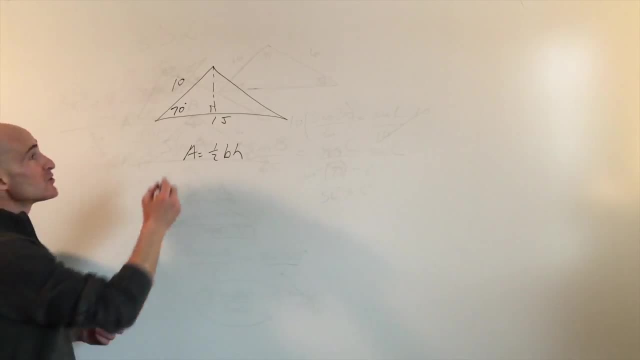 What we can do is we can do: sine of 70 equals h over 10. So sine of 70 degrees equals h over 10.. By cross multiplying we get h equals 10.. H equals 10 times sine of 70.. 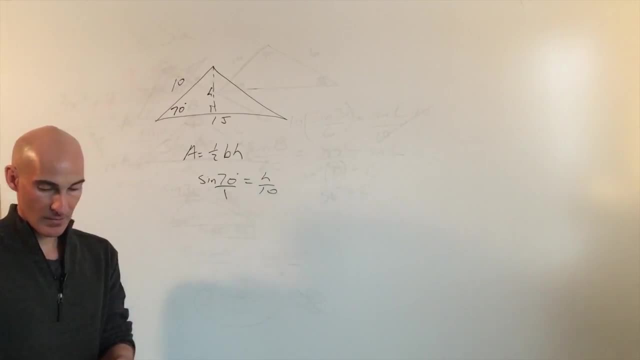 So let's see what that is: 9.4, we'll round And now we can do 1, half the base, 15 times the height, 9.4.. We have the area of the triangle, So let's just write that down. 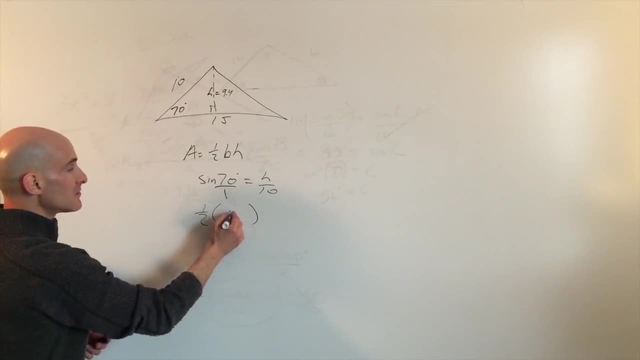 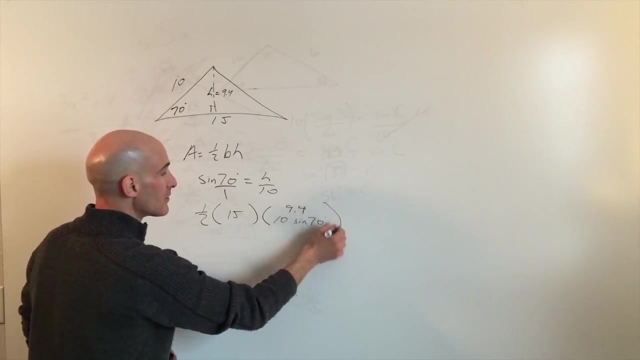 1, half the base, which is 15 times the height, which is 9.4.. But where do we get the 9.4 from? It was 10 times the sine of 70.. So what I want to point out here is that this is one way to find the area of the triangle. 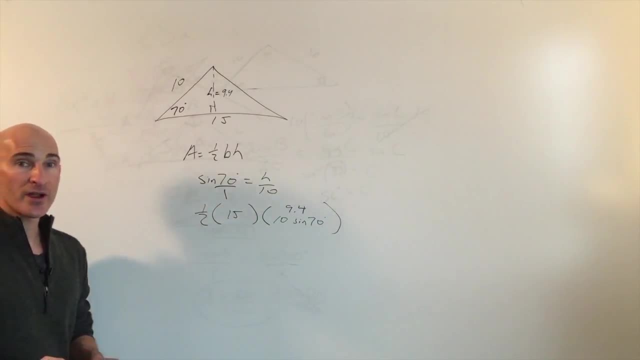 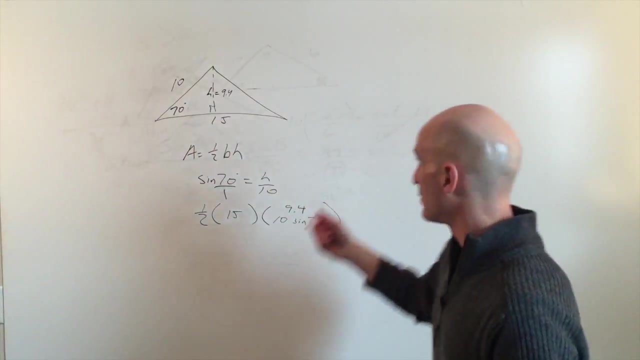 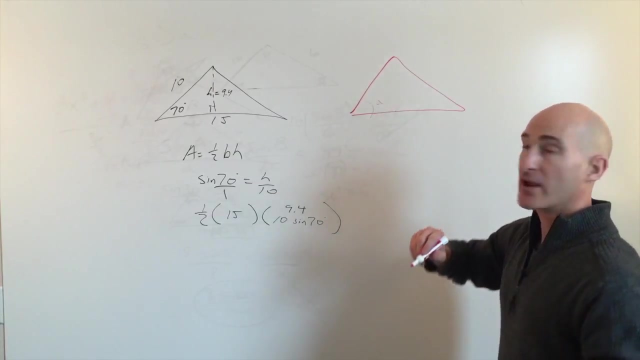 The other way to find the area of the triangle is to use this formula right here that I'm going to show you. next, Let's go over here to this side So say you know this angle. I'm just going to write A for angle A. 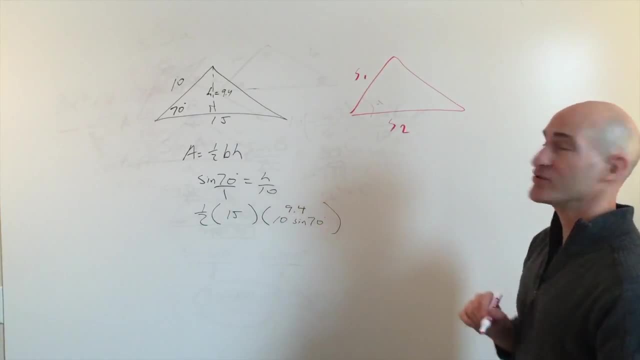 And you know this side. Let's say we'll call this side 1 and this side 2.. If you want to find the area of this triangle, all you have to do is do 1 half times side, 1 times side, 2 times the sine of the included angle. 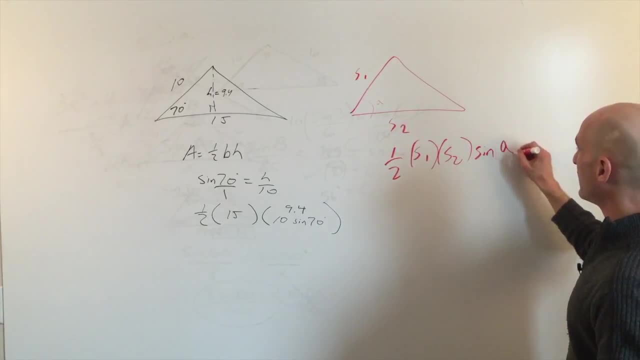 Included means in between those two sides. So sine of angle A. Okay, right here, And that's it. That's the area of the triangle, So it's very easy. So if you have side angle, side, The angle is in between two sides. 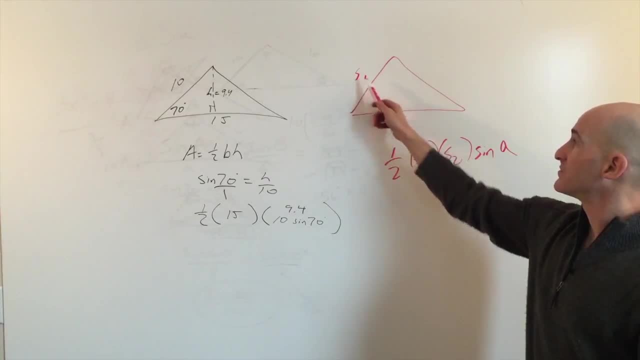 All you have to do is do 1, half the two sides multiplied together, times the sine of the included angle, And you got it. So a quick example would be like this: Say this is 30 degrees, I like 30 because 30 is easy to find the sine of. 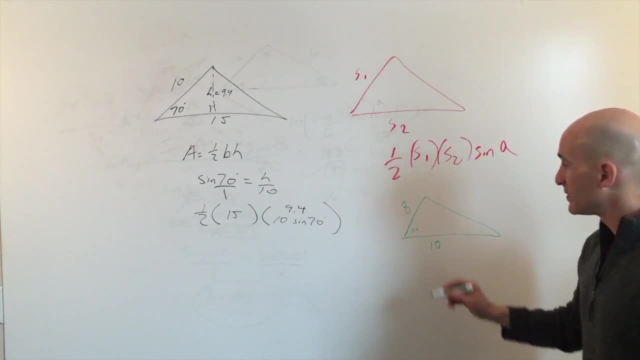 And then you've got 8 and let's say this is 10.. So very simply, it's going to be 1 half 8 times 10 times the sine of 30 degrees. So if you multiply all those together, you get 1 half times 8 times 10 is 40 times the sine of 30..